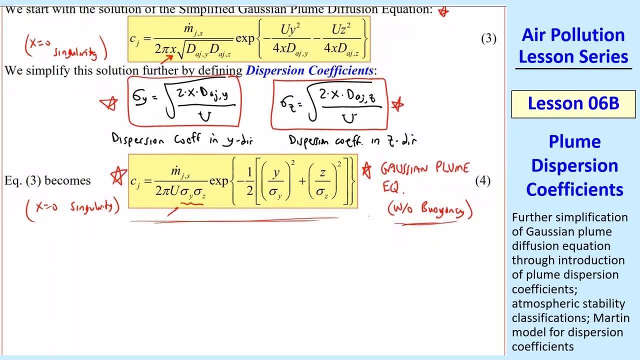 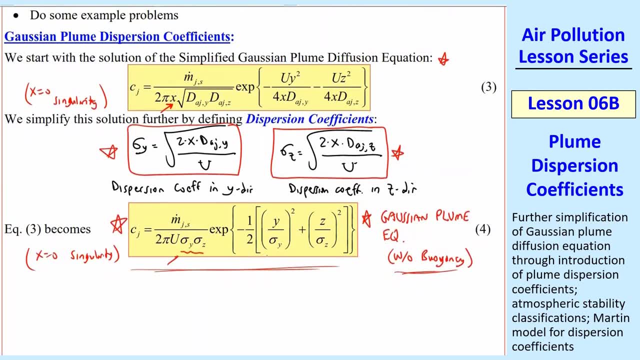 All we've done is change the equation to one in which we have these so-called dispersion coefficients instead of the diffusion coefficients d aj y and d aj z. We now have sigma y and sigma z. We still have to calculate those. so these are unknowns, and I'm going to show you how to find those. 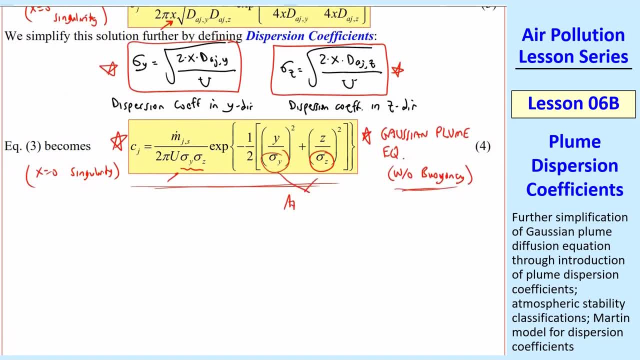 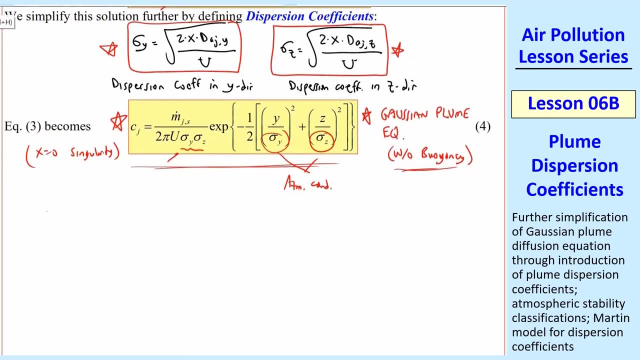 based on the atmospheric conditions. So these come from the atmospheric conditions where the plume is putting out its air pollution. A couple other comments on here about this. equation 4 is valid for x greater than 0. So you can't use it at x equals 0, because it's infinity, it's a singularity. 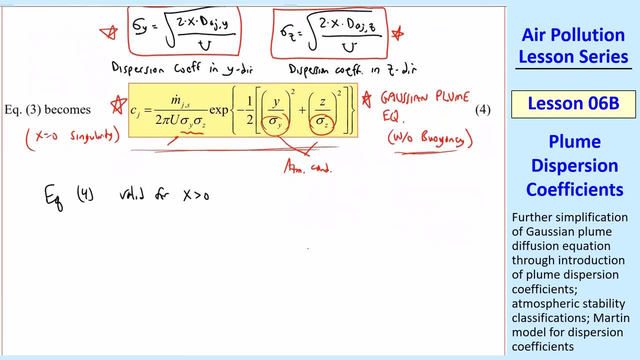 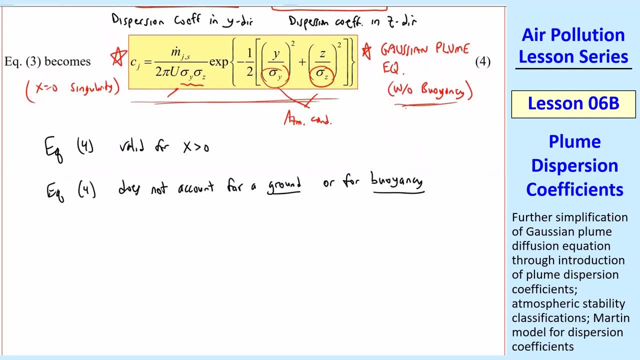 And then anything downstream of the plume, downwind of the plume, you can use it. And then also, this model does not account for the ground or for buoyancy, as we already said up here. So we haven't taken that into account yet. 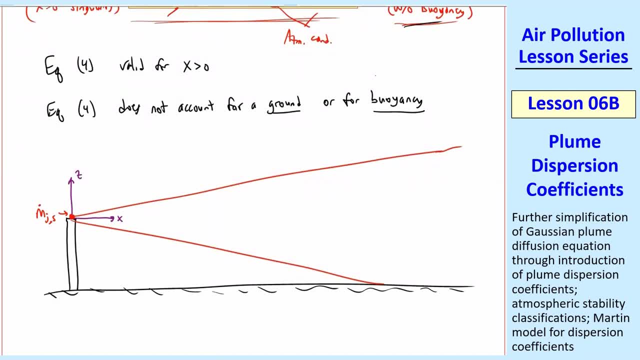 So we're neglecting buoyancy. We have the plume just going horizontally. There's no hot plume or cold plume that would go up or down, And we put the source right at the top of the stack then, And then this plume spreads as you move downstream. 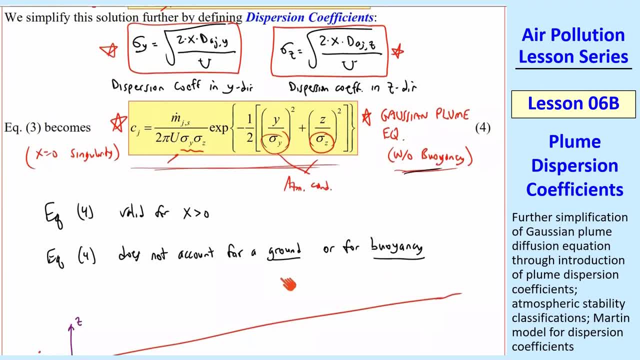 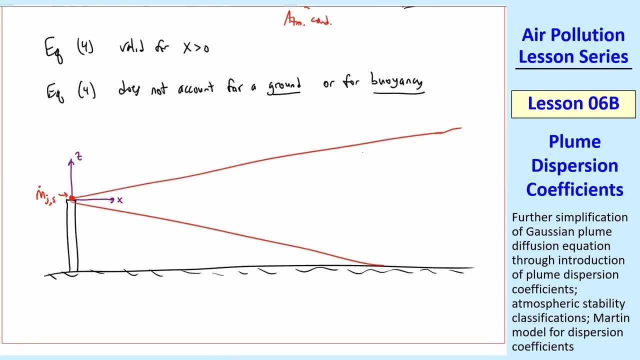 We don't even know there is a ground in this equation. It does have no idea that there's a ground. So in real life though, this will eventually hit the ground, Of course it's a Gaussian. so when you say hit the ground, you have to talk about some kind of small number. 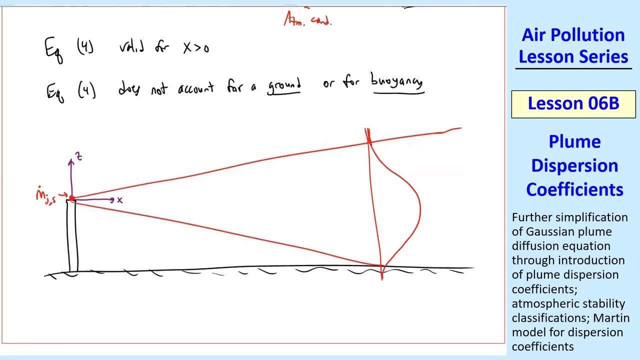 It is a Gaussian, It never hits the ground. Technically this goes to 0 at infinity plus or minus. But at some point you do a reasonable small number and say the concentration is below a certain value when it, quote, hits the ground. 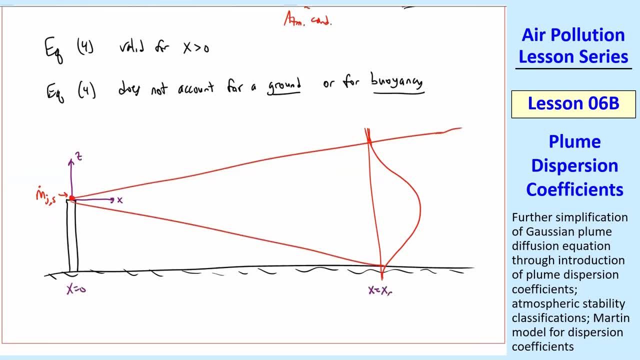 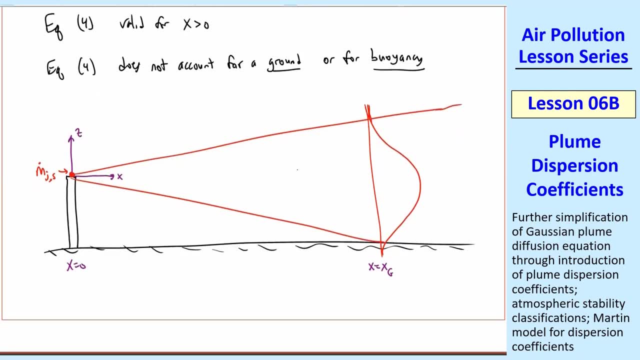 This, of course, would be x equals 0. And we'll call this x equals x sub g. for where it hits the ground, We don't know where that is yet. I'll do some analysis with that later, But for now let's just say that equation 4 is valid for 0 less than x, less than xg. 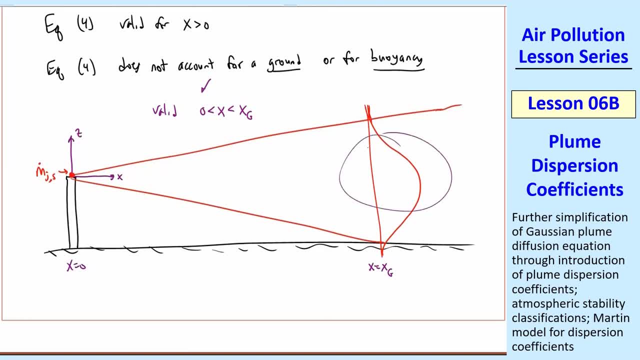 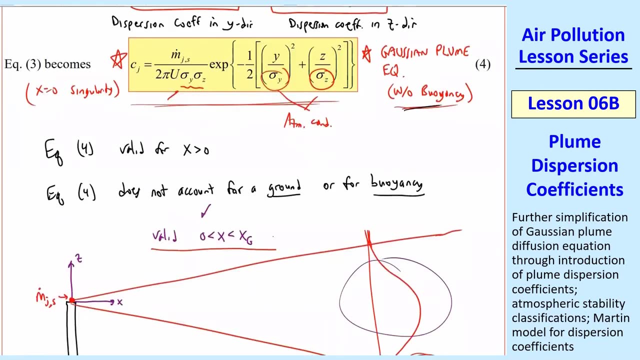 Once it hits the ground it'll still be valid up in this region. But anything below, after it hits the ground in this region, we have to talk about that and treat that a little more special. So in summary, this equation 4 is useful for Gaussian plumes without buoyancy and for the range 0 to x to xg. 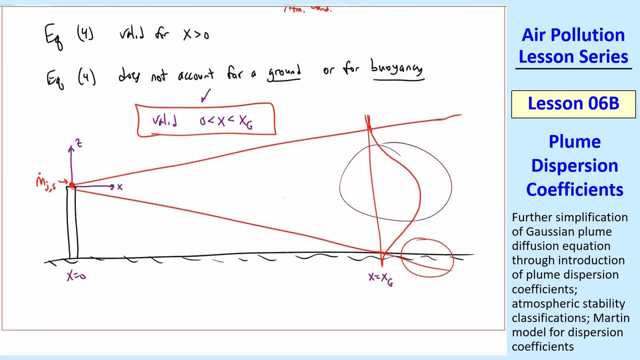 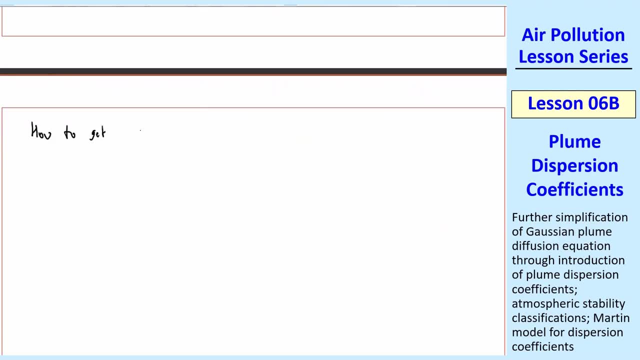 plus all the other assumptions and approximations we made before, such as steady, constant u, etc. All right, So now the problem remains: How to get these dispersion coefficients, now sigma y and sigma z? And the answer is: empirically. 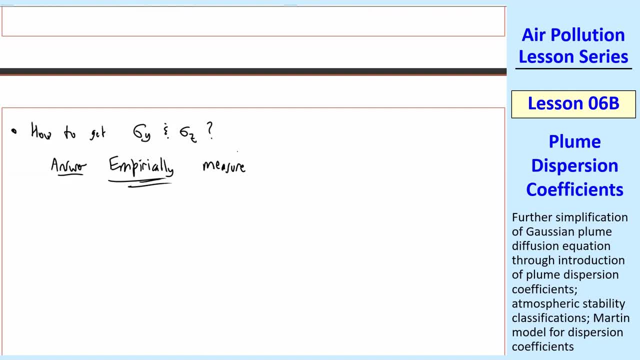 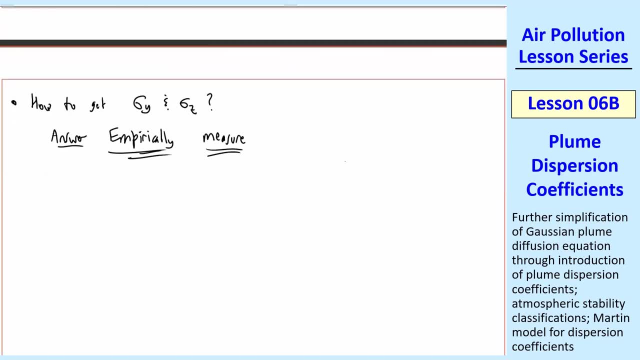 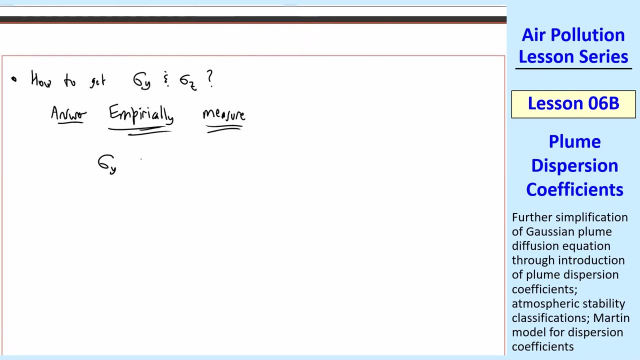 In other words, we have to measure these plume diffusion coefficients in various wind and weather conditions. Meteorologists have done this. These are too complex to figure out analytically, So you can do computer simulations or you can do actual experiments. So the ones we're going to be using are old values based on some experiments that were done many years ago. 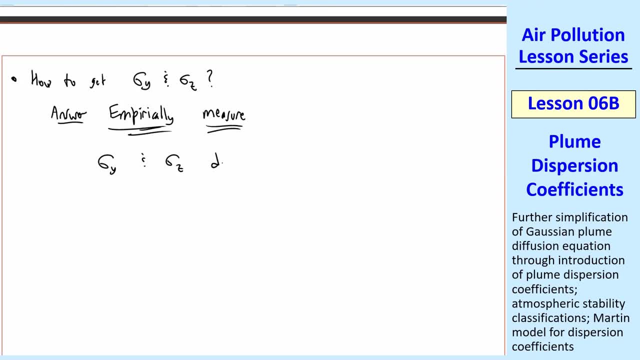 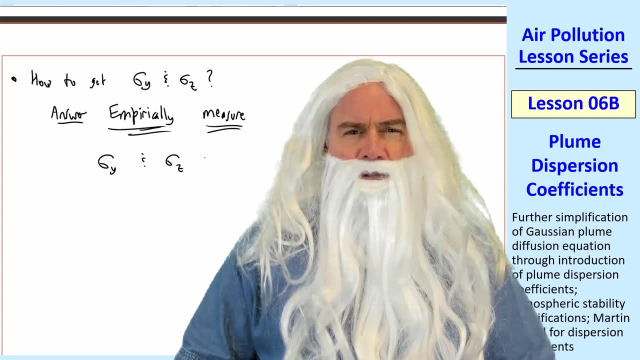 In fact many decades ago. But they're still useful. The atmosphere hasn't changed. The behavior of these plumes hasn't changed in decades, as long as you describe them well. Yeah, just because things are old doesn't mean they're useless. 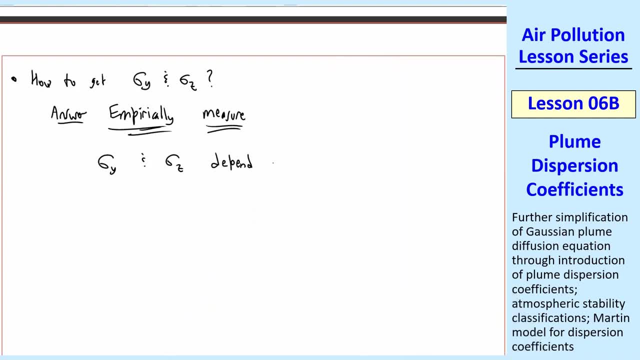 Yeah, you tell them Pops. So these sigma y and sigma z depend on many things: the terrain. So do you have forest? Do you have a city with lots of buildings? Do you have mountains, hills, etc. Of course they'll depend also on wind speed. 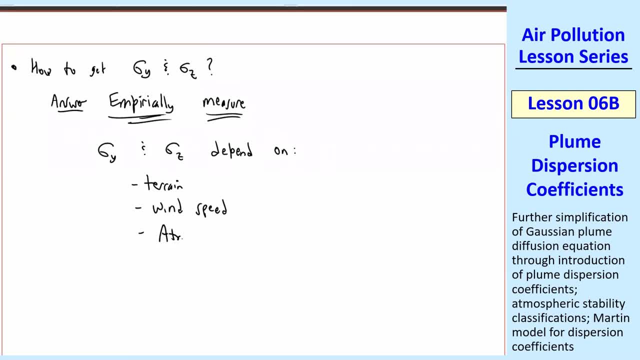 So wind speed will determine how fast things diffuse, Something we've already talked about quite a bit: atmospheric conditions, such as lapse rate and solar radiation. How high is the sun above the horizon, Things like that, Of course. the x from the source, the distance from the source where the plume is being created. 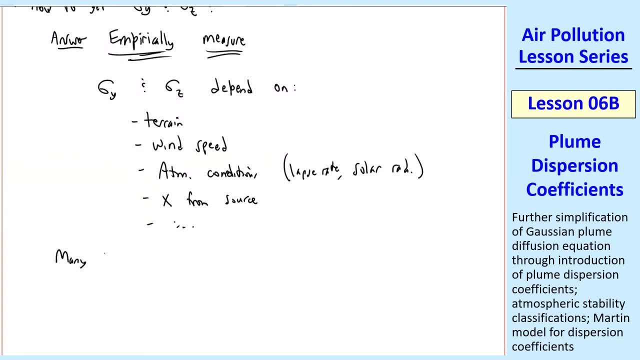 And some other stuff that we'll look at, And there are many possible models that you can use And some are very complex models. If you really get into this, you will use some more complex models, But one very simple one that we will use for everything we do in this course is called Martin's model. 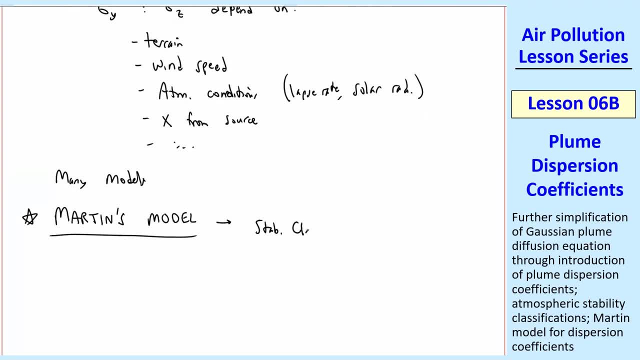 The way this works is you determine a stability classification And this is capital A, B, C, up through capital F, And these range from A is very unstable- to F is very stable. So something like temperature inversion conditions would be F. Something very unstable would be when you have, like we talked about before, with lapse rate. 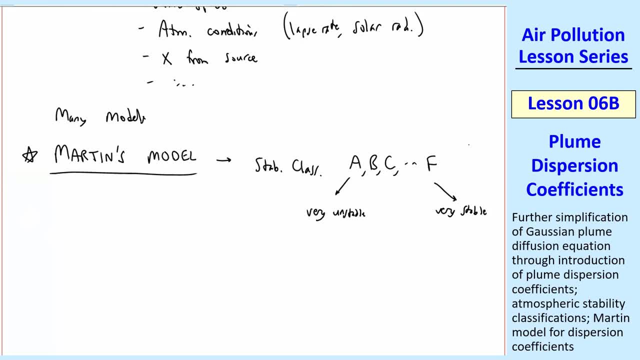 a very large lapse rate in the red zone to the left of that neutral as we talked about previously. So Martin's model is actually fairly simple. It's sigma y is equal to some coefficient A times x to the B power And sigma z is some coefficient C x to the D power plus F. 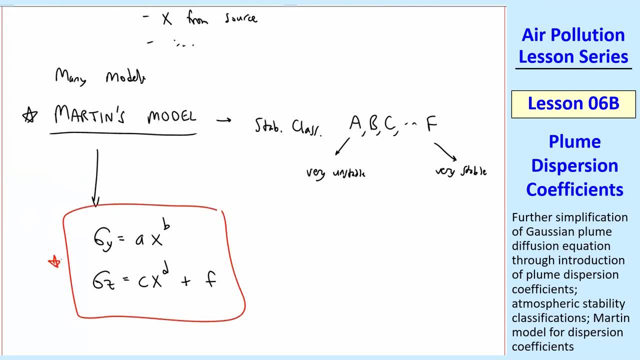 And so these are nice, simple equations. The only difficult thing, And students have made numerous mistakes with this, So I'm warning you that these are engineering equations And so x is in kilometers, But when you get your answers, sigma y and sigma z are in meters. 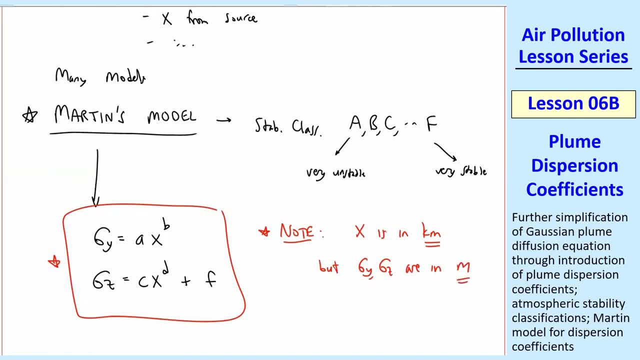 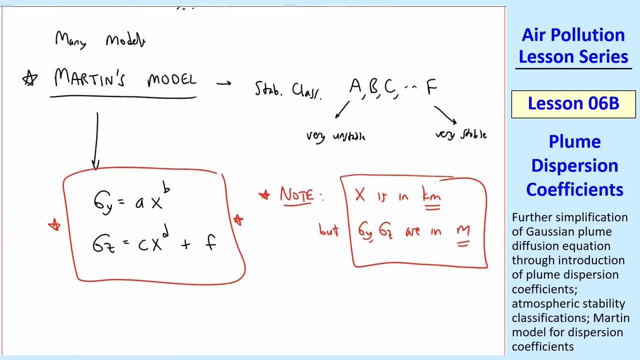 These are engineering equations which mean you just have to put in the values exactly in the proper units. And the proper units here are x in kilometers, And then you'll get your results in meters. So as long as you know that and are careful with that, you should not have a problem. 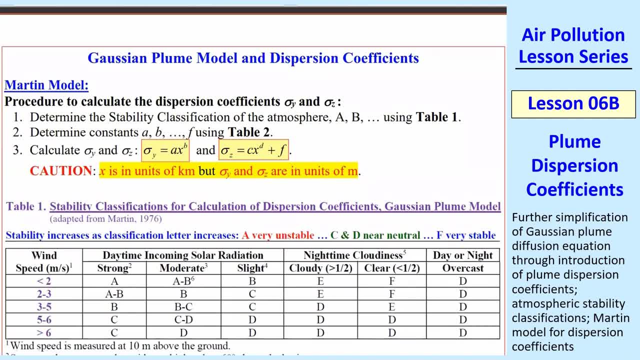 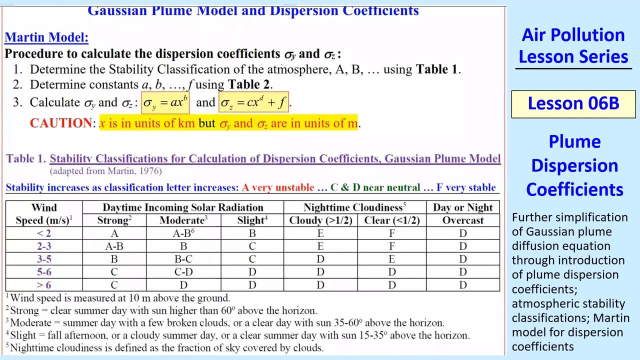 So here's a table And this is also on your equation sheet, So we're going to be using this quite a bit. Here's the procedure for the Martin model, And the goal is to determine sigma y and sigma z. And let's not get lost in what we're doing here. 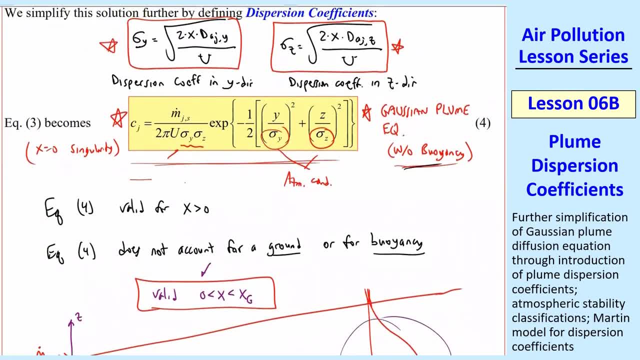 The reason we need sigma y and sigma z is once we have that, we can calculate the C- j at any point in this plume, Any x, y and z. So you're at some point here near the ground at some x location. 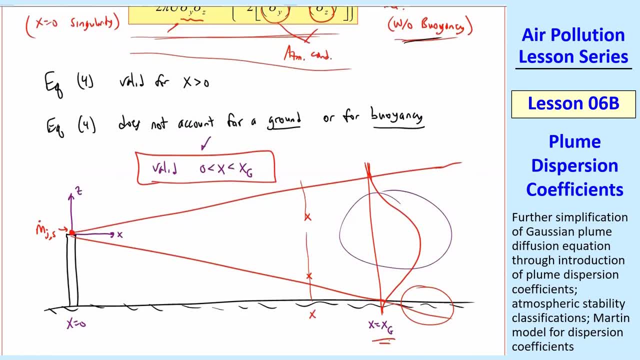 As long as x is there, As long as x is below xg and above zero. So you're in the plume And you want to know. you know, maybe I'm standing here And I'm breathing this air And I want to know: am I breathing harmful air at that point? 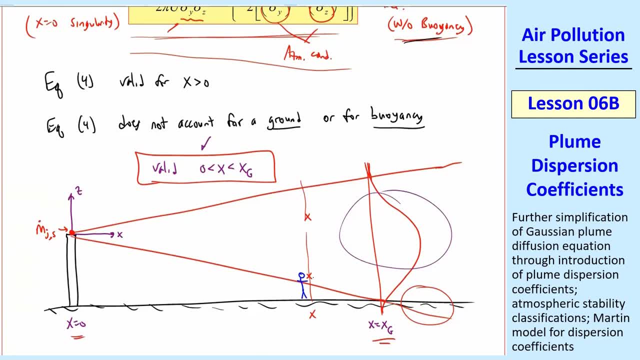 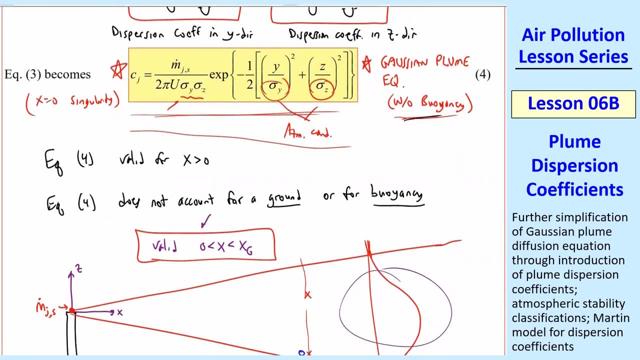 And y is into the page. So at some x, y and z location I can use this equation to calculate my C, j, But I have to know sigma y and sigma z. I will know everything else in here, assuming I know the source, strength, m, dot, j s, the wind speed, etc. 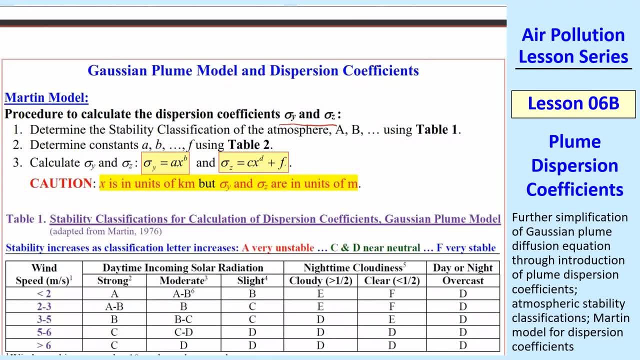 So that's our goal. So, step one, determine the stability classification of the atmosphere, And those are the letters a, b, etc. Using table one. Then we determine constants a, b, etc. Using table two, And then we use these equations which I rewrote here, retyped here: 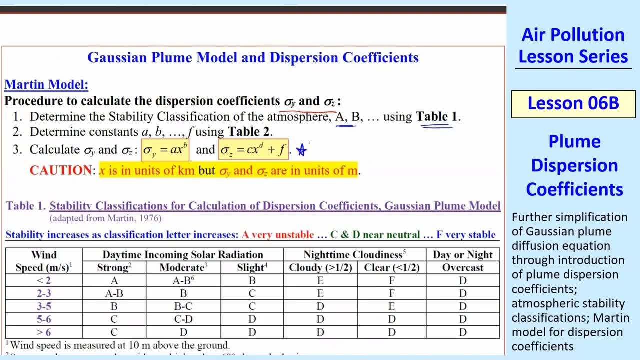 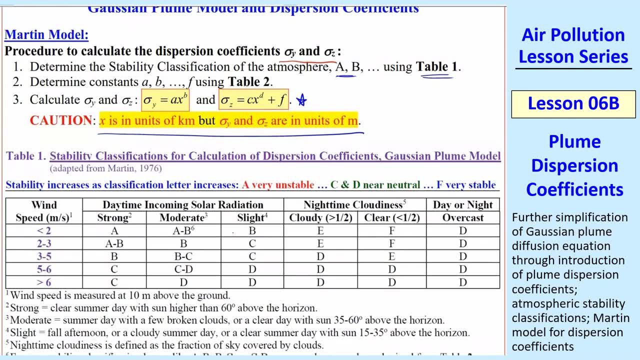 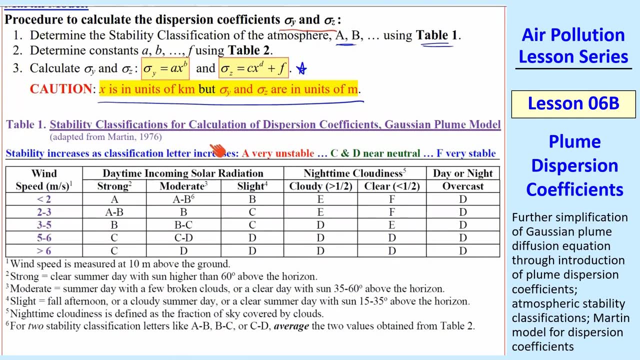 So we use these equations to get our sigmas. And again I caution that x is in units of kilometers But sigma y and sigma z are in units of meters. So here's table one: Stability classifications with Martin's model. And I'd comment here: stability increases as classification letter increases. 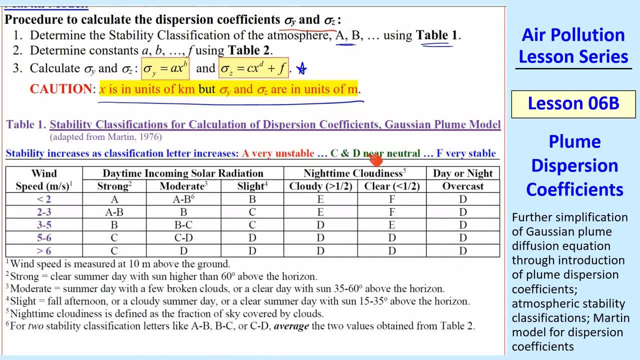 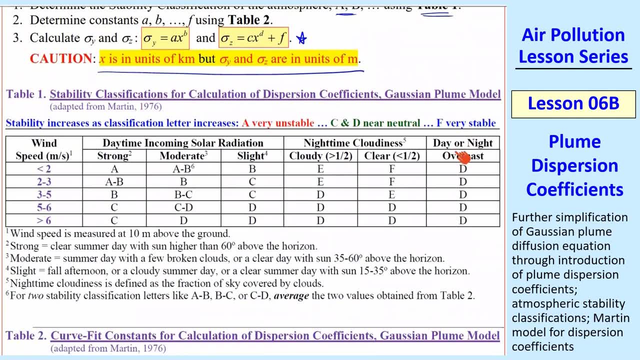 So a goes from very unstable or red to nearly neutral, around C and D, And then very stable is blue, f, the same color coding that we had before, And they also depend on the wind. These wind values are in meters per second, And then these footnotes are very critical. 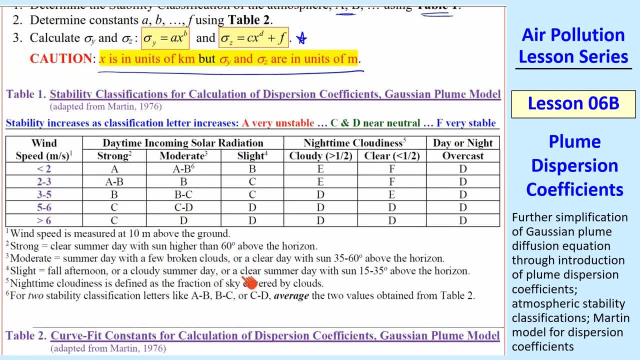 On exams and homeworks and quizzes. you look for hints on how I describe the day. For example, let's just pick one: A clear summer day with the sun higher than 60 degrees. So I tell you that the sun is at 80 degrees above the horizon. 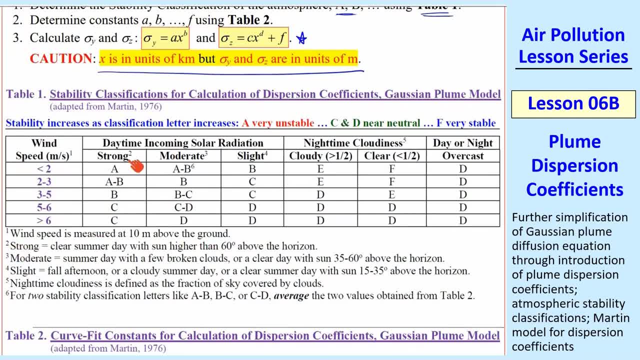 It's a clear summer day, And note two. So that's here strong, And then, depending on the wind, this would be an a or an ab, a, b, c or a c, Depending on how strong the wind is. 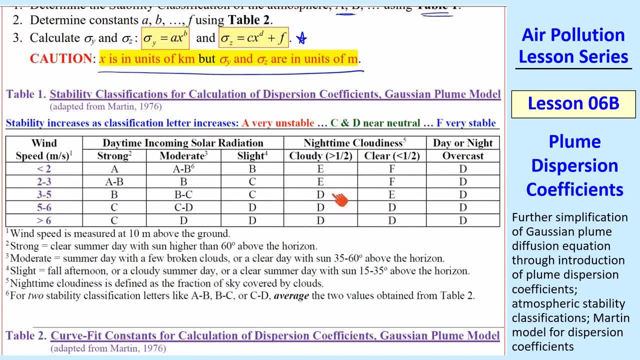 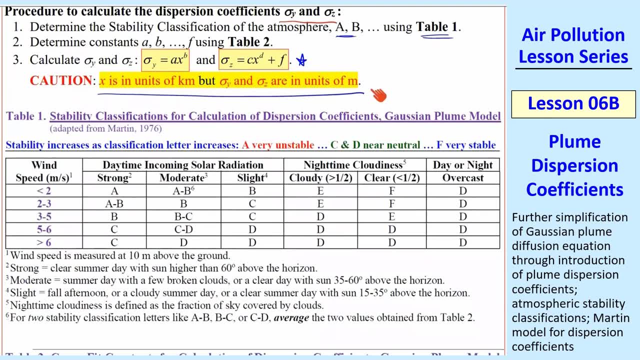 And then you use these other descriptions to figure out whether you have a, b, c. So the bottom line from this first step is you determine a classification- a- b. Some of them are kind of in between a and b And b in between b and c. 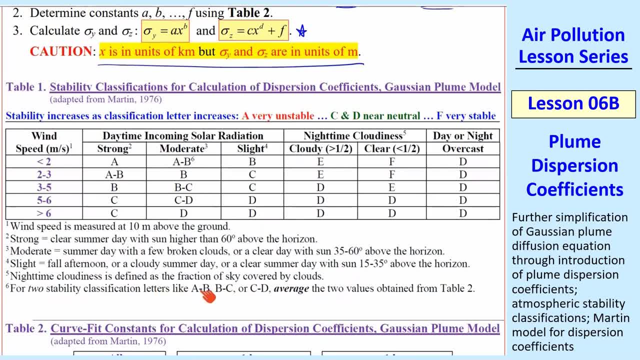 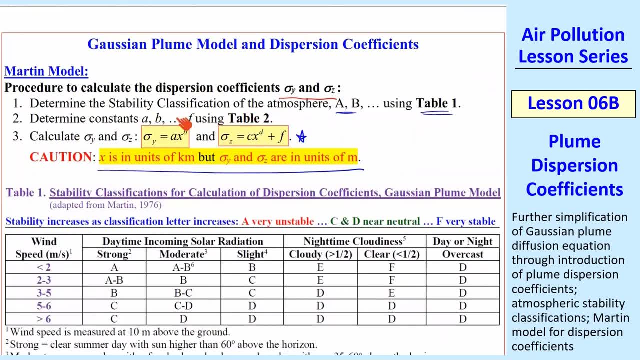 There's one footnote about that. For two stability classification letters like a-b, b-c, you average the two values from table two, Step two. use table two to find these a, b, c values. Now notice there's no e. 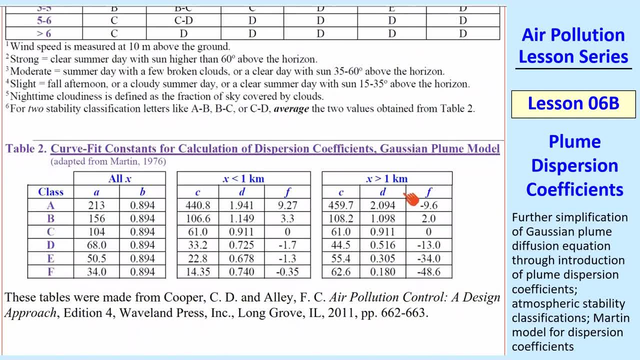 They skipped e so that you don't confuse that with e as a exp, the exponential function. So class a, b, c, d, e, f. And then here's your coefficients for all x, a and b, A and b: are these values for all x's, depending on the class? 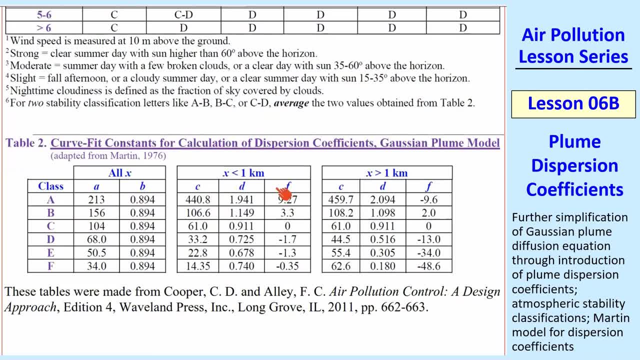 They depend on class, of course, but they don't depend on x For c, d and f. however, they depend on x If x is less than a kilometer or if x is greater than a kilometer. use these values for that. 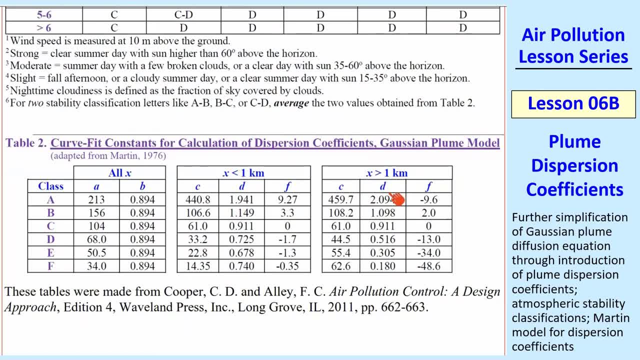 You use these values when x is greater than a kilometer, And so, once we have those, you decide which letter you have, and then you figure out which of these coefficients you have, And if you're at, for example, a, c, d, your a would be the average of these two. 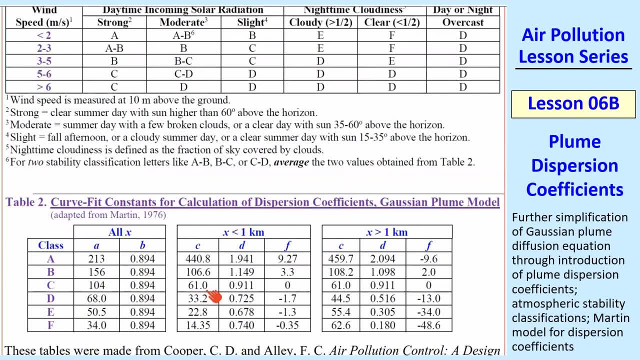 Your b would be the average of these two. Your c would be the average of these two if your x is less than a kilometer. Your f would be the average of these two if your x is greater than a kilometer. So you get the idea. 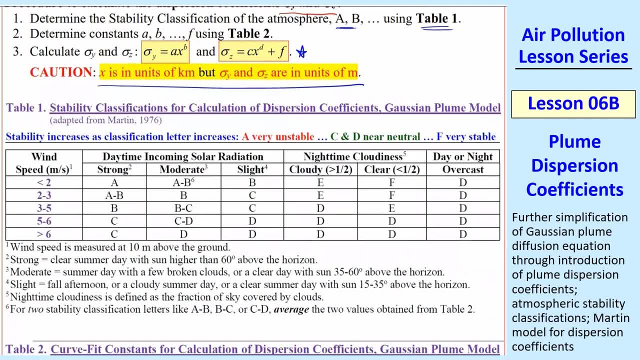 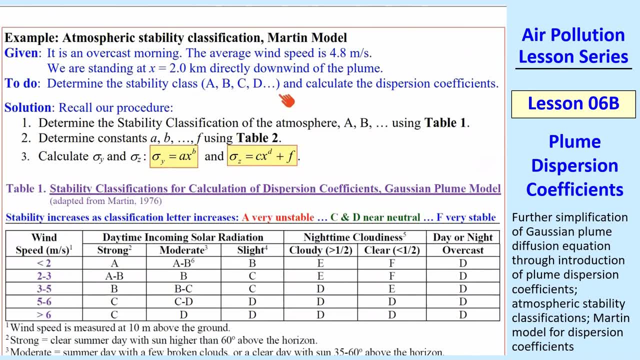 And then, finally, step three is to calculate these dispersion coefficients. So let's do a quick example, And you'll have to do this as part of calculating all the plumes that we do. from now on, We'll be doing a number of plume calculations once we add the ground and we add buoyancy, etc. 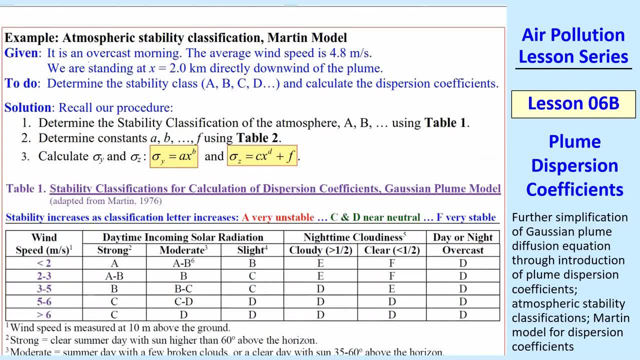 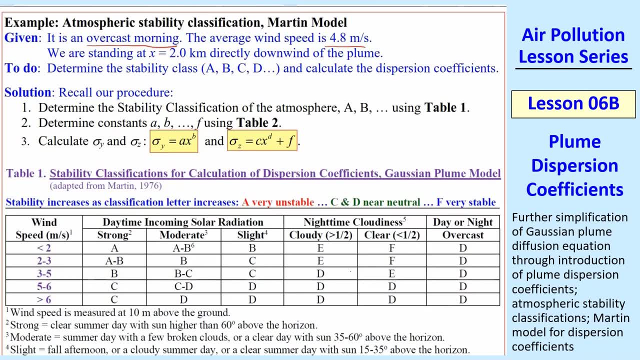 So let's look at this example problem. We have an overcount And here you see the flow along the plane of a picture of this wind speed. So I didn't tú check the stress in advance last morning. Okay, that's a big hint. 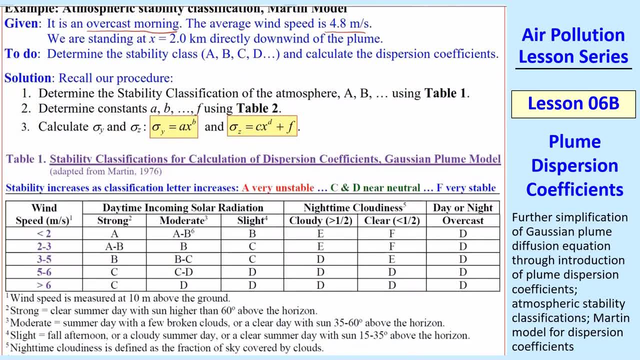 The average wind speed is 4.8 meters per second. So you have to look through this table one to do Step 1, determine the stability class. So I'm looking for the word overcast And the wind speed is 4.8, so we're in this wind speed. 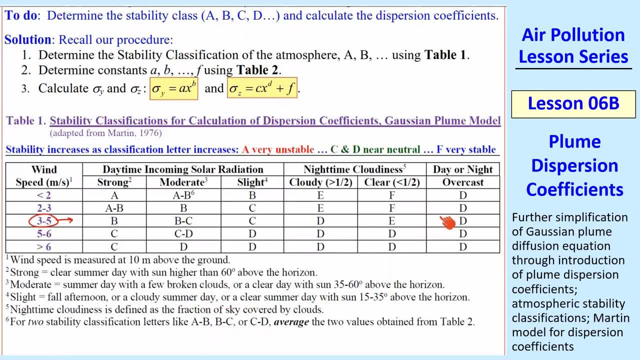 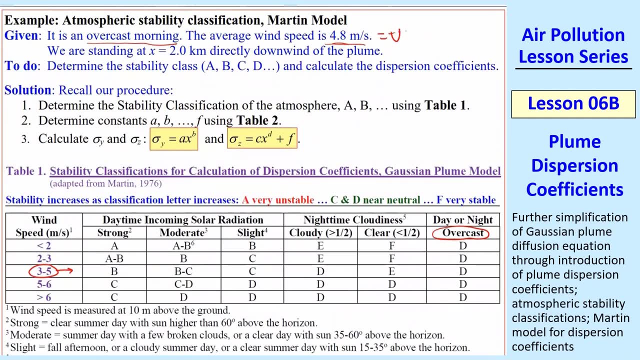 So we're going to go across and look at these footnotes. I don't see anything about overcast here. say, all right, that's my key. my hint: overcast day or night, so it doesn't matter if it's a day or night, overcast three to five meters per second, because we have 4.8, that's our u and so this will. 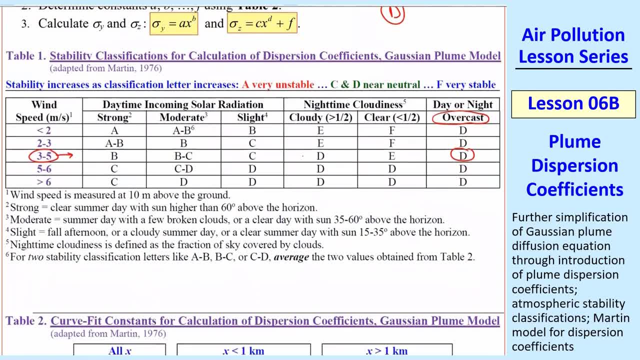 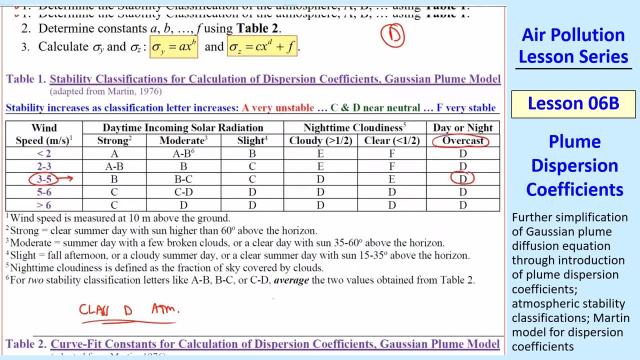 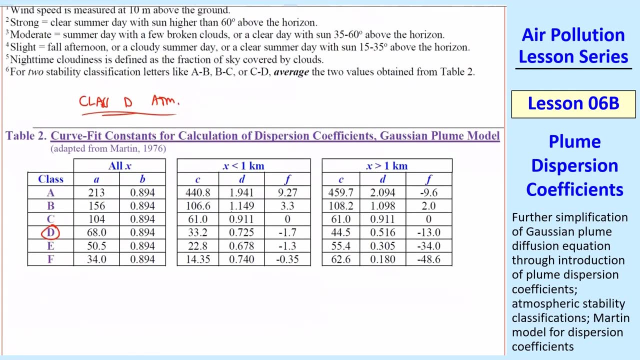 be a d classification letter. so this is a class d classification. we just call it class d, atmosphere, according to martin's model. once we know that, step two is to determine those constants. so that's easy. once we know that, we just go to d and i'll just circle all the values we have now. what's our x? 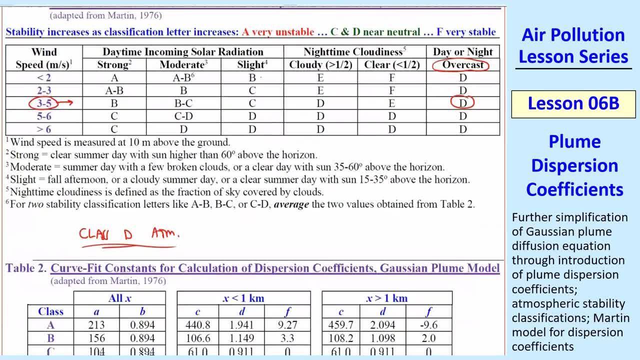 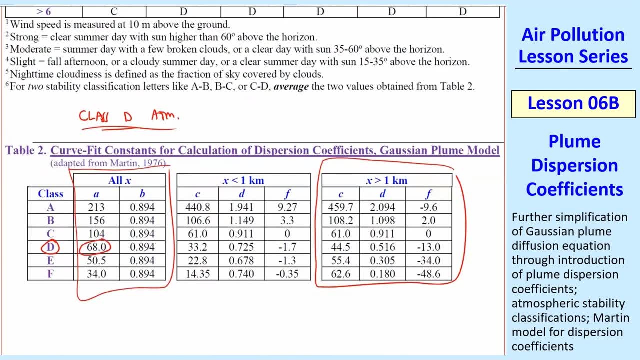 our x is 2.0 kilometers, which is greater than one kilometer. so we use this table and this is felt for all x. so our a is 68, our b is that, our c is that, our d is that and our f is that value. 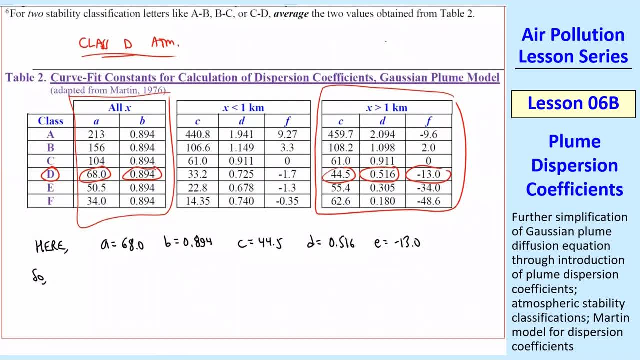 so let's just summarize. so i just wrote down all those coefficients and now we can calculate: sigma y is equal to a, x to the b, plugging in all these coefficients and our x in kilometers. this is the only tricky part. then you don't worry about units, you just get your answer. in meters. sigma y is 126.37 meters. 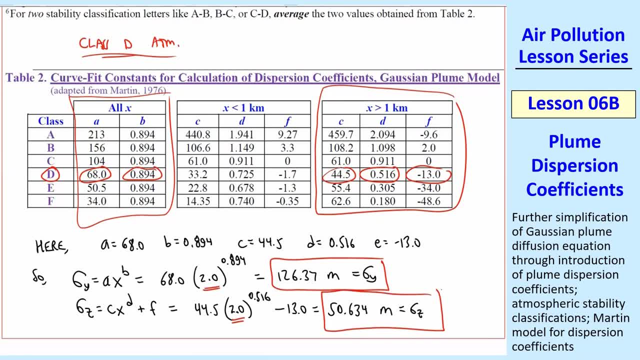 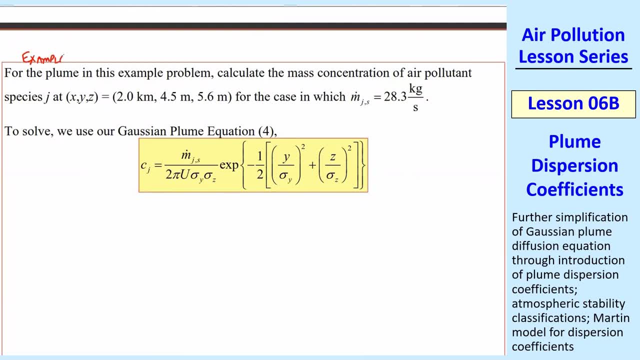 and sigma z is 50.634 meters. so that's our sigmas, and then i'll do another example here. for this final example i want to do: what we really want to do in these kind of problems is calculate the mass concentration of the energy. and then we're going to calculate the mass concentration of the energy. 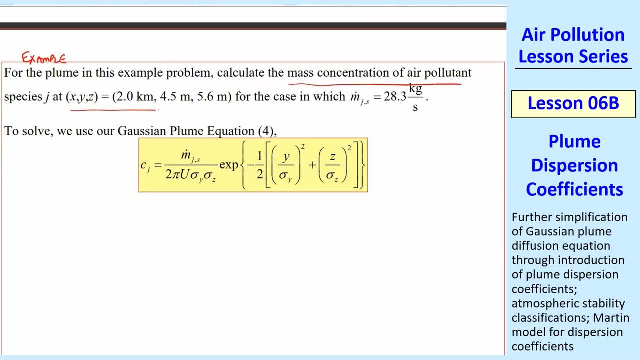 of the air, pollutant of some species, j, and i give you x, y and z, so some location downwind of the plume, and i have to also give you m, dot, j, s, so that's the source, source strength, and so if that's known, then 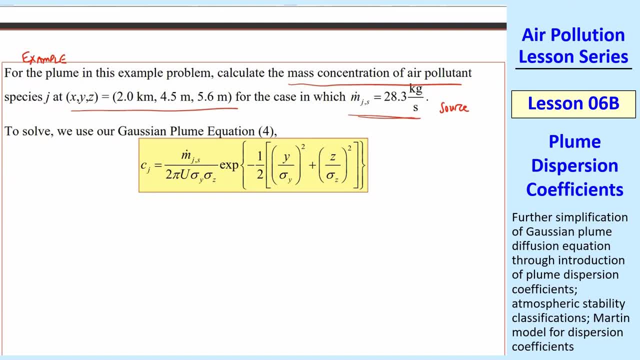 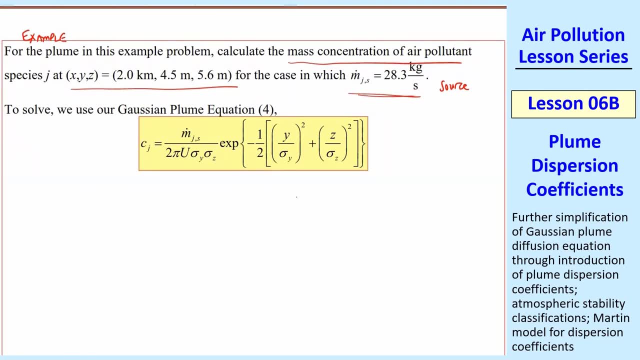 we should be able to calculate. we have everything we need in this equation and so, again, we're assuming the buoyancy in this plume and we haven't done anything with the ground yet, but just out in the air, somewhere where there's this plume, we can plug in this equation and generate our final answer. 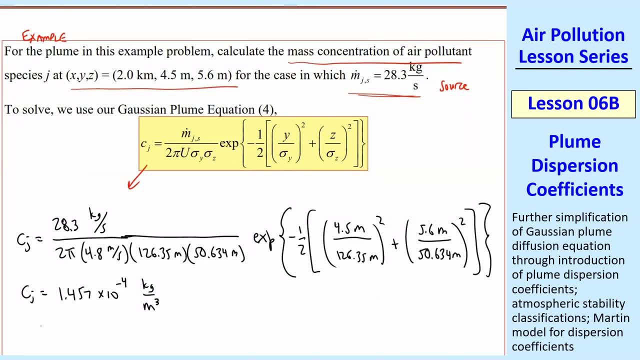 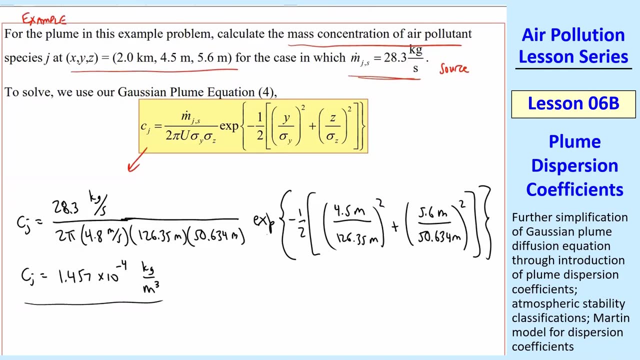 i plugged in all the numbers and here's our final result, in units of kilogram per meter cubed, which is a mass concentration. but usually you do that in milligrams per meter cubed, so i'll have to convert. but i just wanted to point out a couple things here. when you do any analysis in any course, 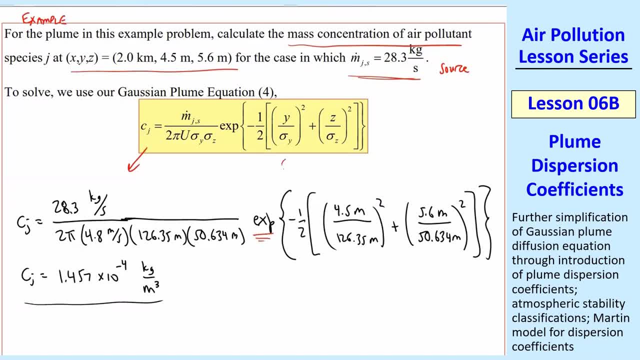 anything you're doing with an exp function, everything within these brackets, everything in here, has to be non-dimensional, has to be no units and all the units must cancel because exp of anything, what any of the units that you're doing with an exp function is going to be non-dimensional. 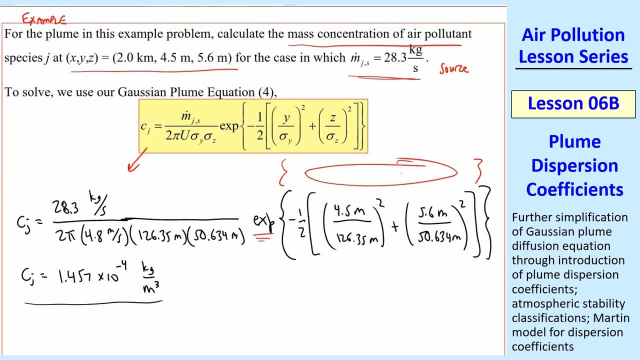 because exp of anything, what any of the units that you're doing with an exp function is going to be non-dimensional. anything is in there, inside the brackets, has to be no units and you can see that the meters here cancel. so this is dimensionless. the units here, the seconds, cancel, so we get kilogram per meter cubed. 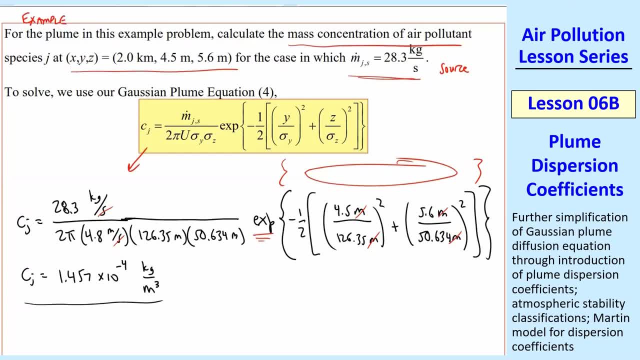 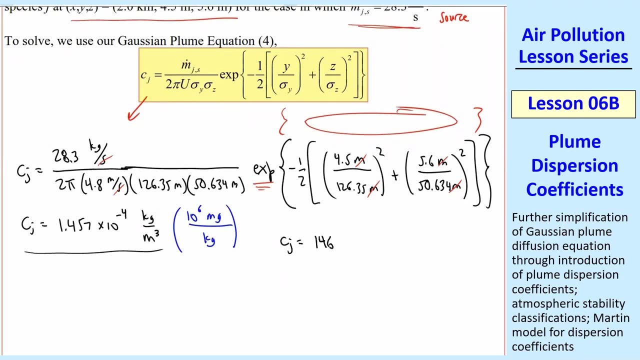 and, like i said, we usually don't give mass concentrations in these small numbers, with kilogram per meter cubed, but rather in milligrams per meter cubed. so 10 to the 6 milligram per kilogram, and that gives us then our final result, which we would write: cj is equal to three digits 146. 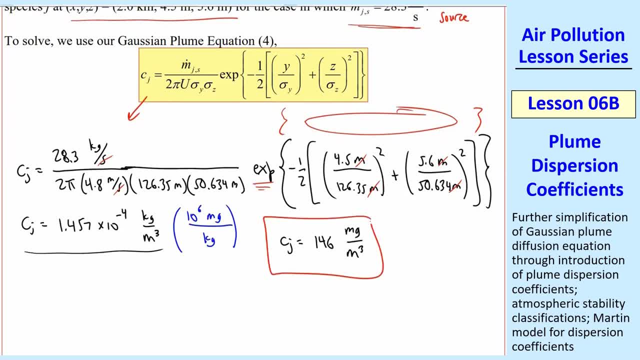 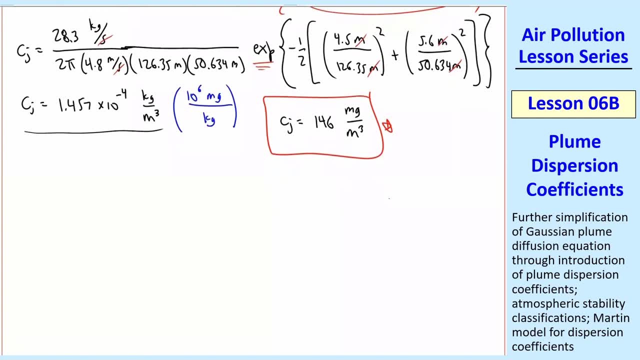 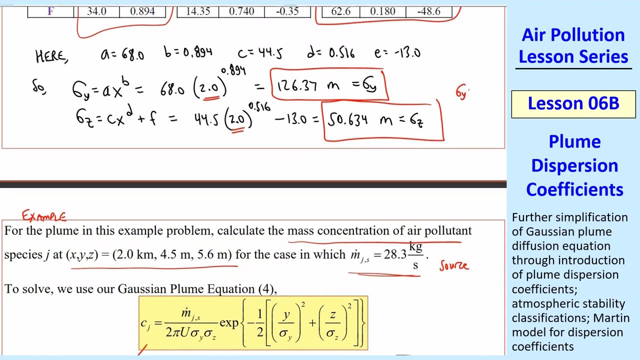 kilogram per meter cubed, which is our prediction. and now you can compare that with pel or with the nax, depending on what this chemical is. i just want to make another comment here, based on these dispersion coefficients that we calculated. notice that here sigma y is greater than sigma z. so what? 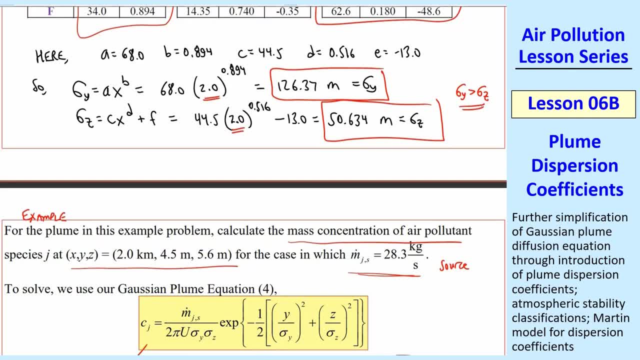 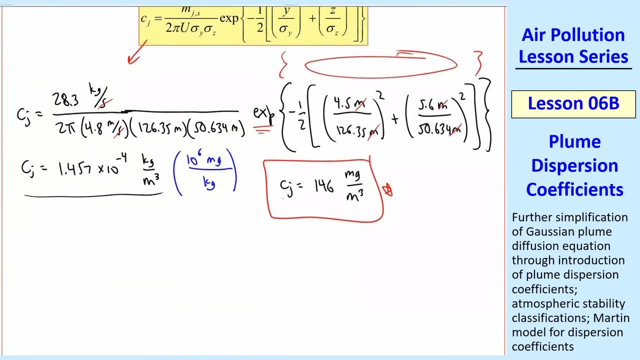 does that mean? that means that this plume is spreading more rapidly in the horizontal or y direction than it is in the vertical or z direction. so that means that this plume is going to spread more. So this is a somewhat stable plume because it's spreading more rapidly horizontally than 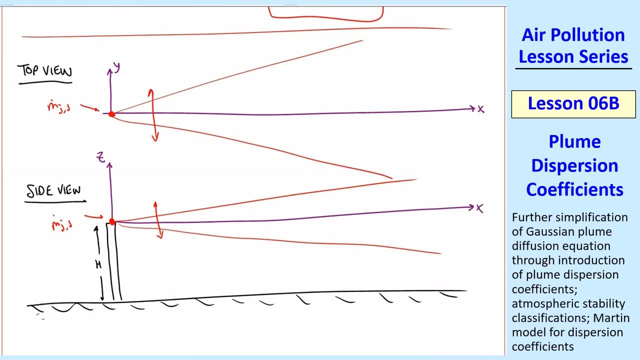 it is vertically, This might be moderately stable kind of a plume. Therefore, what are we looking at? We're at some x location. This is x equals zero, and we're at x. that was given 2.0 kilometers. So let's just suppose that's here at x, equal 2.0 kilometers, And 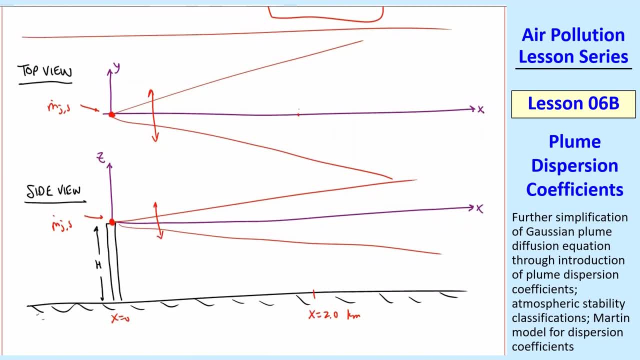 we're not on the center line in this problem, but we're at a y value. So on this top view, we're at some y value. that's here, and we're at some z value that's a little bit further than that. These may not be the same scale vertically and horizontally with the y's and 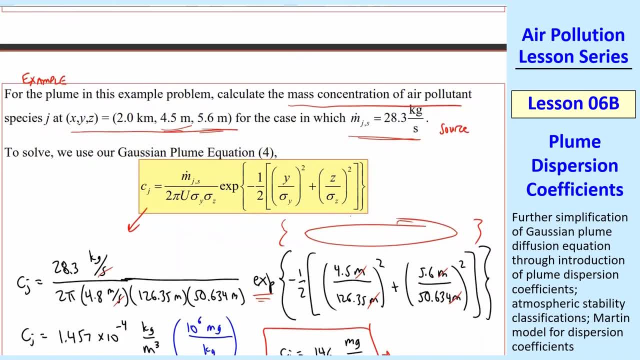 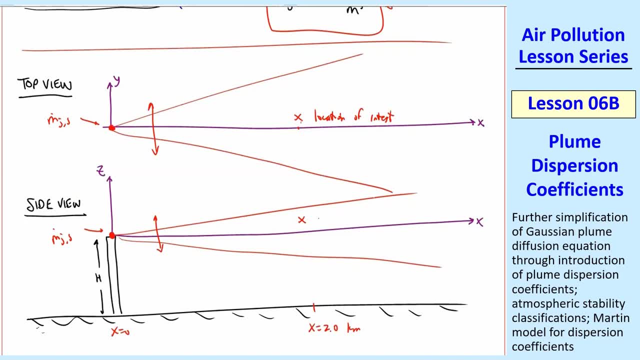 the z's, but our y was 4.5 meters, Our z was 5.6 meters, So they're at this location. So this is the location of interest in the top view and the location of interest in the side view, And we see that the plume is spreading more rapidly horizontally than vertically. 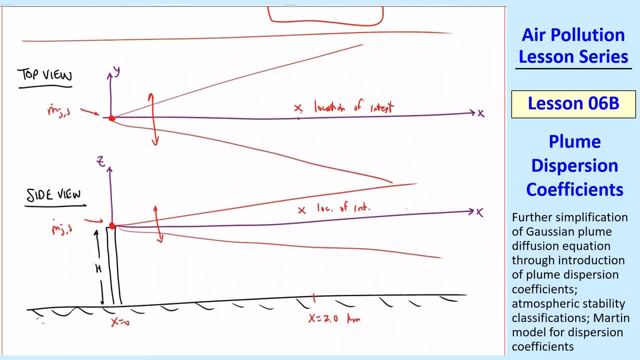 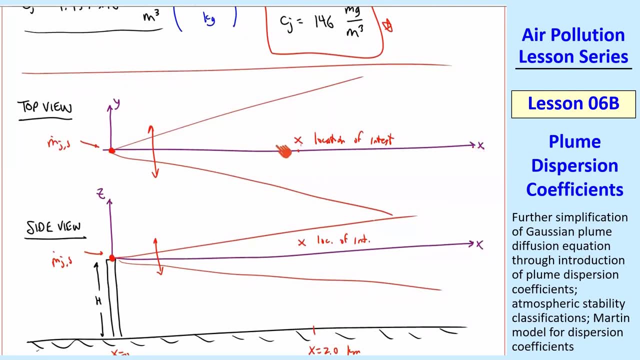 like I said. So you will have some practice with these plumes. And one other thing I wanted to comment: notice that these plumes are generally symmetric across x, So it doesn't matter if you're going to the left or the right or the top or the bottom of the plume, And you can see. that's. 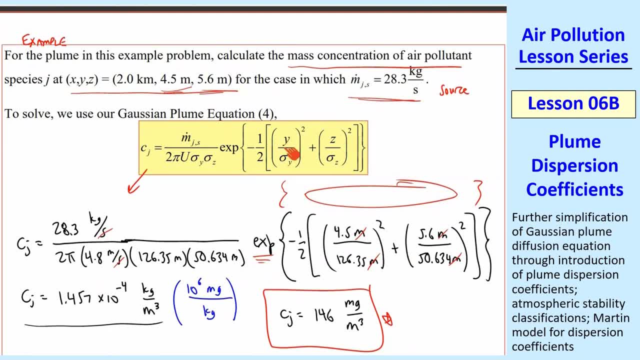 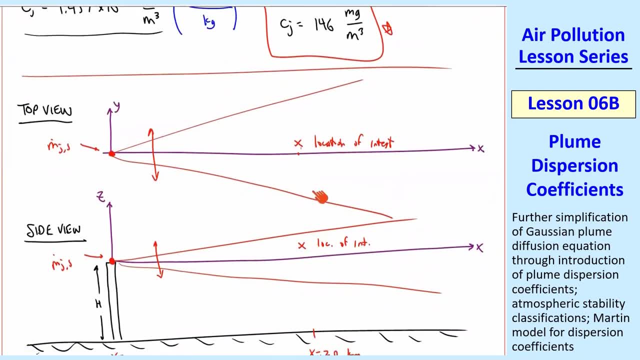 true here, because whether z is positive or negative or y is positive or negative, it's not going to matter, because those terms are squared, So you really only have to calculate half of it. But you should be able to calculate cj at any given location, as long as you know. 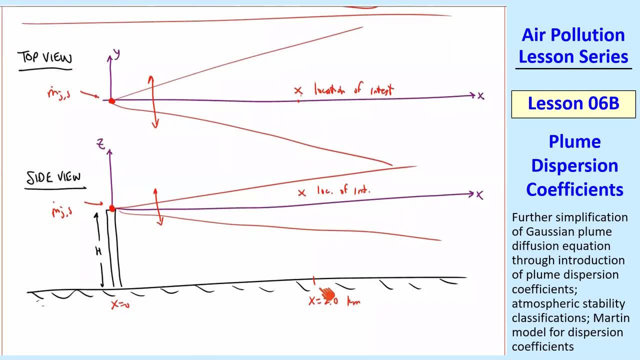 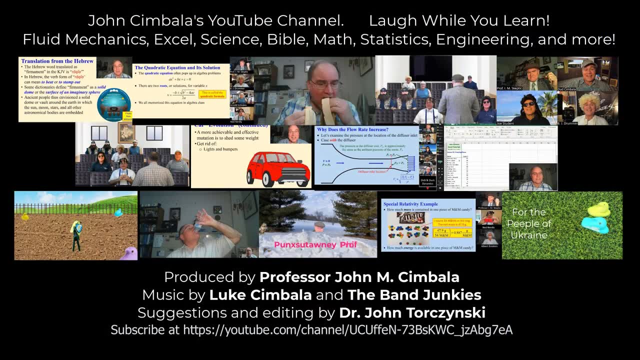 the length, the location and you know what the kind of plume you have, And then later we're going to add buoyancy and we have to deal with what happens when this plume gets close to the ground. Thank you for watching this video. Please subscribe to my YouTube channel for more videos.